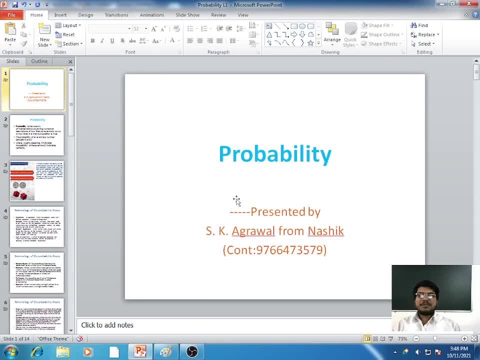 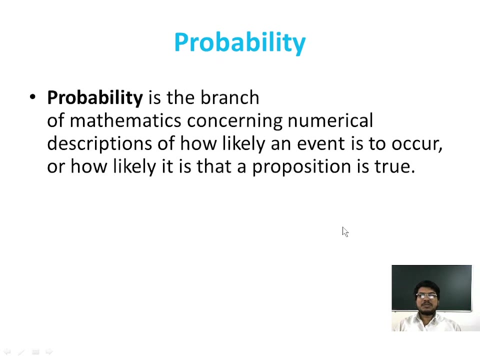 Have a great day, friends. I am Sushant Agrawal here discussing Probability. Now, what is probability? Probability is the branch of mathematics concerning numerical descriptions: how likely an event is to occur and how likely it is that a proposition is true. 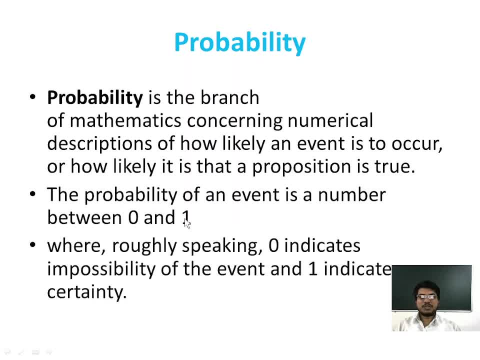 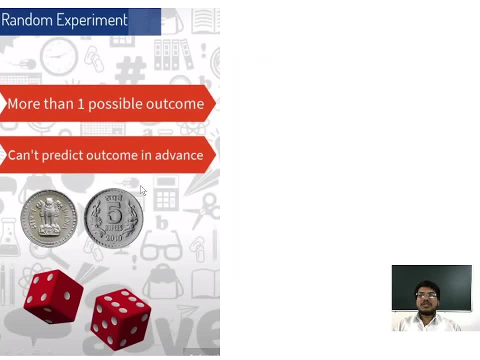 The probability of an event is a number between 0 and 1.. 0 means what Roughly you can speak, that it is impossibility, and 1 means it is what Certainty You can see. we are dealing with the random experiment. What is the meaning of random experiment? These are the two examples. 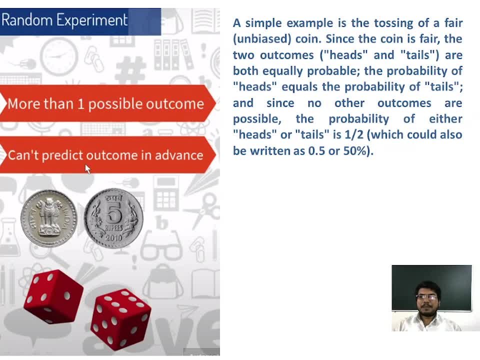 More than one possible outcome can come and it cannot predict outcome in advance. A simple example is the tossing of fair, unbiased coin. Since the coin is fair means there is no we can say any mistake in that coin or we can say it is correct, It is fair, and the two outcomes- heads and 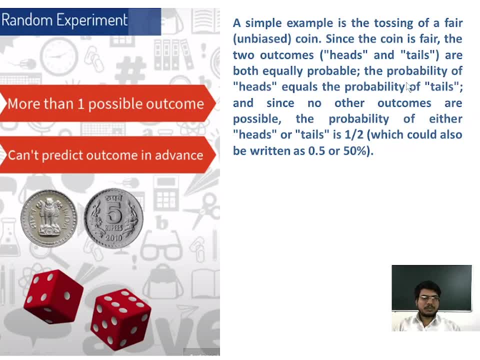 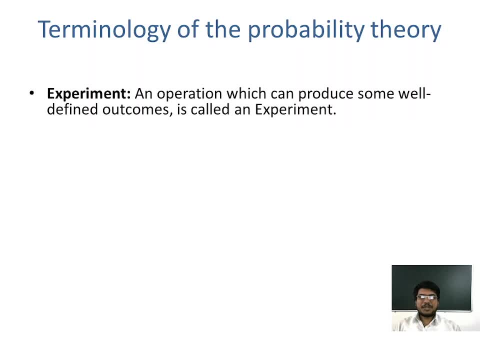 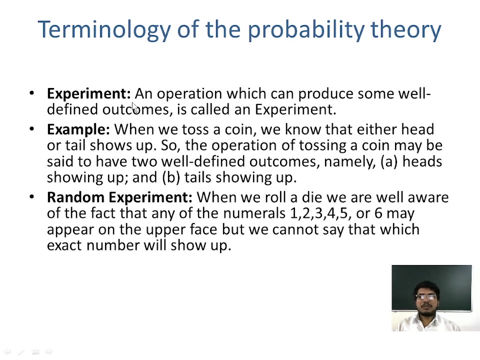 The so called probability errors can be expressed through 45 degrees. The probability alien state. JENN coach has written a new course called Esquire, which is a huge activity which can be defined as 精, a square in XY members, And the main equation here is: нап다 мир지. it's elegant datumوس, There are combinational and it's 1, frames per second. poiI gotij 나와 wird an isolated number by specify to pass as 0.ки has 0.5 or 50%. 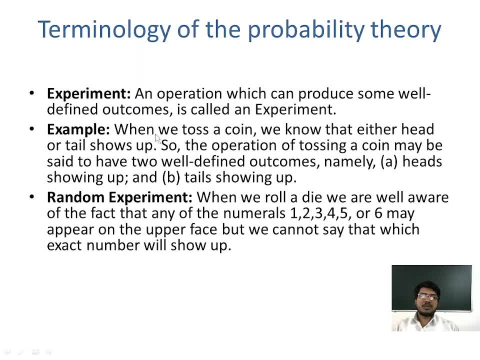 experiments with, we can say, with the coin or with the cards or with the dice. Example: when we toss a coin, we know that either head or tail shows up. So the operation of tossing a coin may be said to have two well-defined outcomes, namely head showing up, and it may be tail showing up. 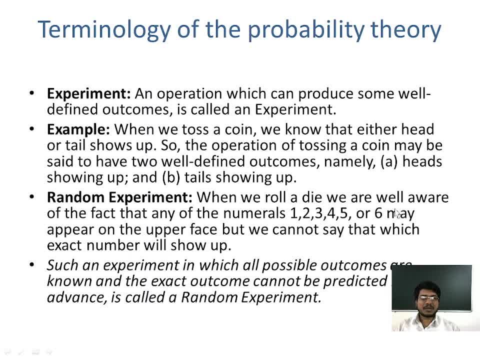 What is the random experiment When we roll a die? we are well aware of the fact that any of the numerals 1 to 6 may appear on the upper face, but we cannot say that which exact number will show up. Such an experiment, in which all possible outcomes are known and the exact outcome cannot. 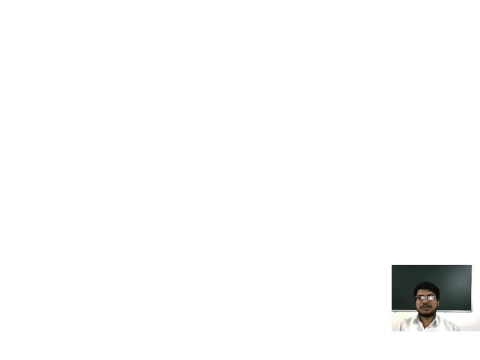 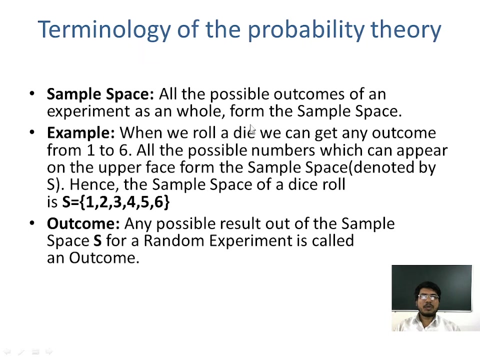 be predicted in advance is called random experiment. Now, what is the sample space? All the possible outcomes of an experiment is a whole form of the sample space. For example, when we roll a die, we can get an outcome from 1 to 6.. 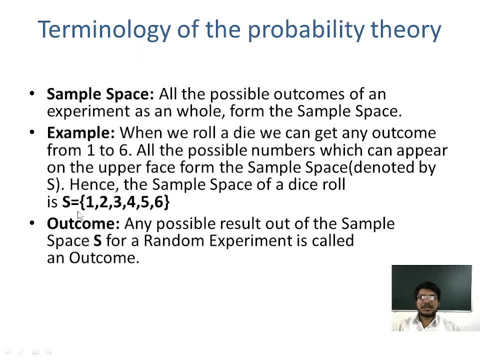 You can see it is in the set. s is equal to set of 1 to 6 numbers. Now outcome: any possible result out of the sample space s for random experiment is called an outcome Example. when we roll a die, we might obtain 3. or when we toss a coin, we might obtain head. 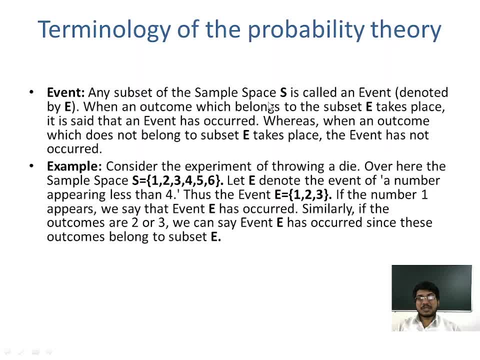 Now, what is event? Any subset of the sample space s is called an event Denoted by e. When an outcome which belongs to the subset e takes place, it is said that an event has occurred, whereas when an outcome which dopes not belong to subset e takes place, the event has not. 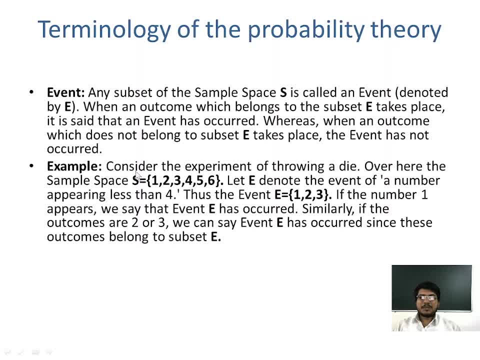 occurred. Now example: consider the experiment throwing a die. So event is there over here. the sample space s 1 to 6 and let e denote the event of the number and we can say that event has occurred. If the number 1 appears, we say that event e has occurred, and similarly, if the outcome 2 or 3, we can say event e has occurred, since these outcomes belong to subset e. 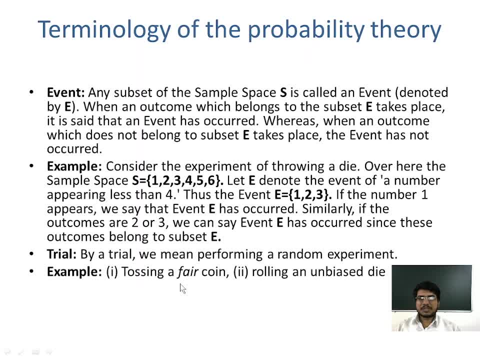 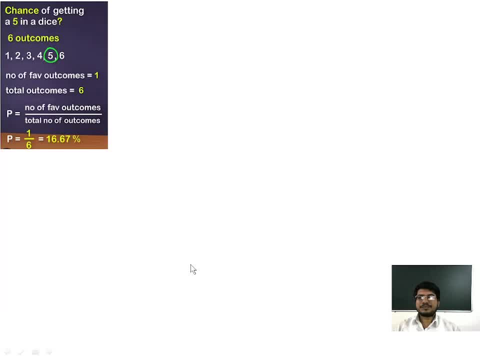 Now what is the trial? By a trial we mean performing a random experiment and example: a tossing a coin or die rolling an unbursed die like that. Now these are the examples. Chance of getting A 5 in a die s. There are 6 outcome about the die s: 1, 2, 3, 4,, 5, 6, like that. 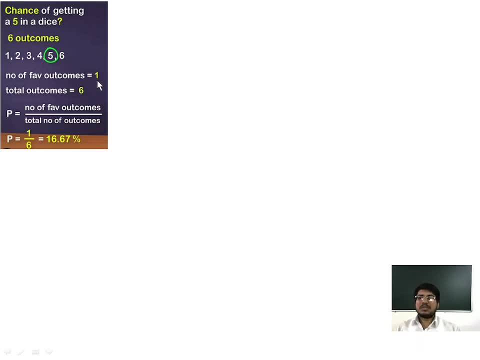 So number of favorable outcomes is 1, that is 5 here, rounded it is, and total outcomes are 6. about the die s. So what is the probability? as per the formula you know, n? a upon n. Last discussion was completed about that. So that is 1 upon 6, it is 16.61 percent. 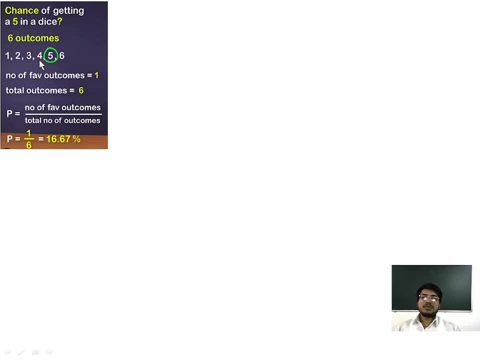 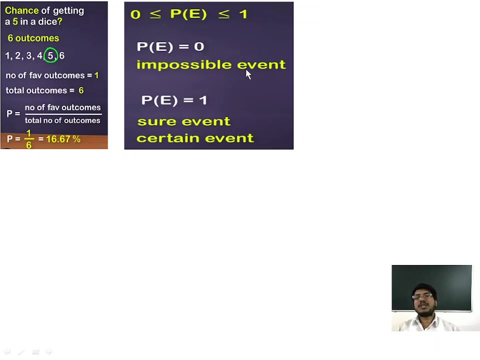 Now, what is the probability for you? What is the chance for getting 4?? Again, same answer will come right: 16.61, 67 percent. Now, second example: this is the meaning given if probability of this outcome is 0. So impossible event. we are saying that so that probability lies between 0 and 1. and if it is 1, probability of that event is 1. that is sure event or certain event. 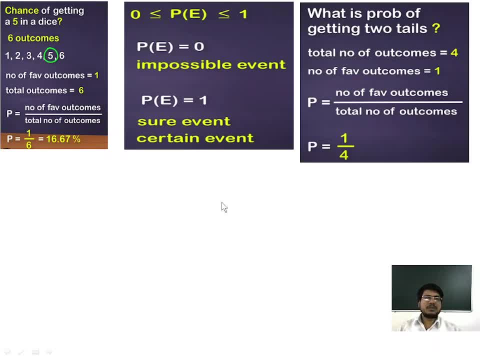 Now what is the probability of that? So probability of that is 0.. So probability of that is 0. So probability of that is 1.. So probability of that is 1.. of getting two tails: okay. so now, total number of outcomes are four. number of favorable outcomes are: 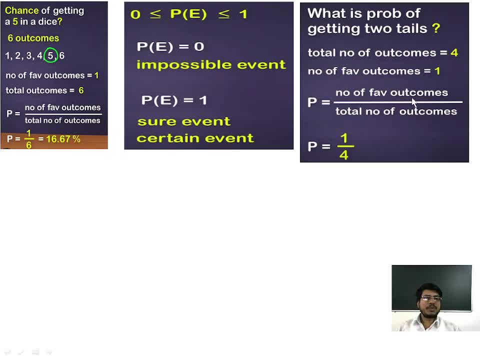 one. so probability is equal to number of favorable outcomes upon total number of outcomes. so that is n a upon n. so n a is in this case one and total number of favorable outcomes are four. to understand the number of favorable outcomes you can write the set here: h comma h, h comma t, t comma h. 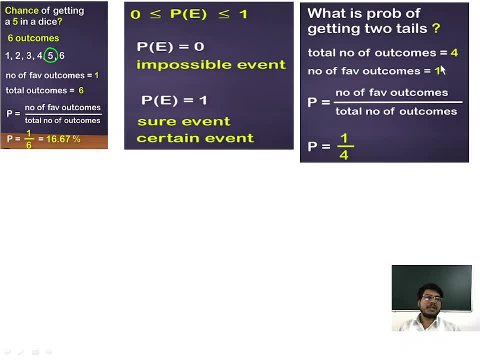 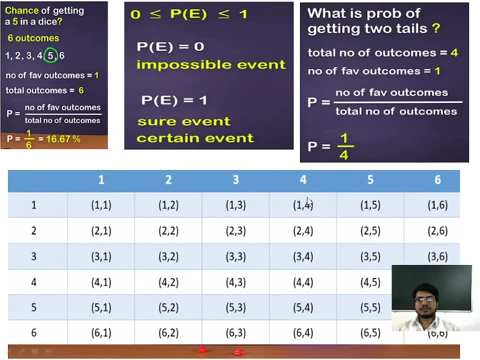 or t comma t, so that t comma t is there and we can say both are tail. so there is a one favorable outcome and total number of outcomes are four. it is the one of the we can say possible number of outcomes due to the two dice. two dice are rolled, so that will be helpful for another. 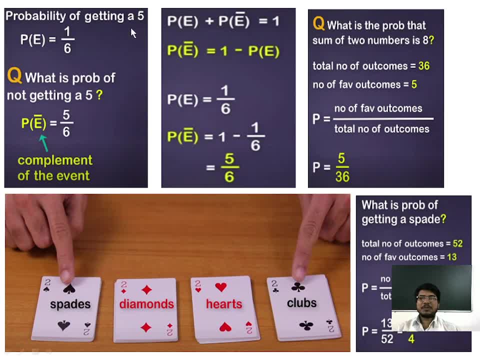 examples now here. probability of getting a five that is one upon six. what is the probability of not getting a five that is one upon six? what is the probability of not getting a five that is a five that is a compliment of the event. you can say probability of a compliment or you: 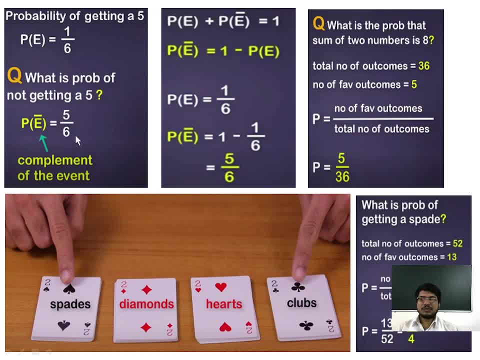 can say e bar, so that is five upon six. you can write one minus one by six and it will become five upon six. so here is the probability of a plus probability of a compliment is equal to one. or you can say: probability of event e plus probability of complement of that is equal to one. 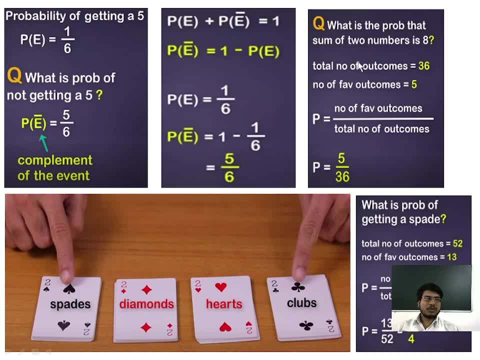 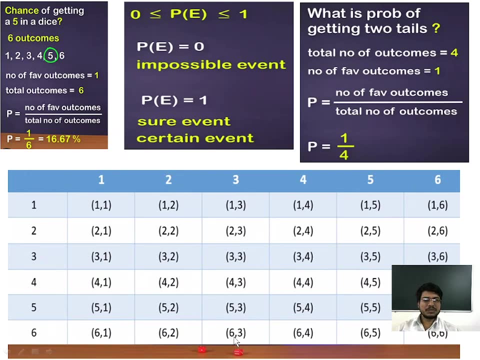 So, in this regard, you can find it out. What is the probability that sum of two numbers is 8?. Total number of outcomes is 36 when you are ruling the two dice Right, And number of favorable outcomes are 5.. How you can count this? Here? you will count this. 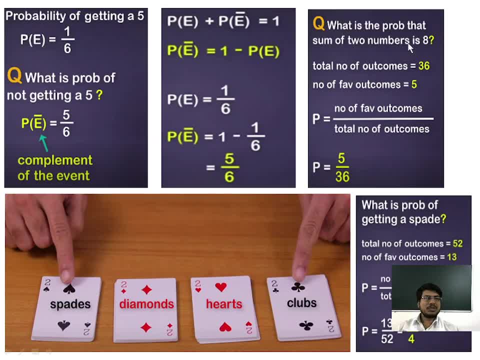 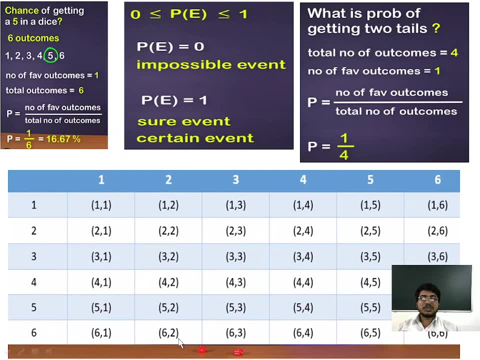 The question is what? Two number is 8. So sum should be 8.. 5 plus 3 is 8. 6. 6 plus 2 is 8.. 4 plus 4 is 8.. 3 plus 5 is 8.. And 2 plus 6 is 8.. So 1,, 2,, 3,, 4 and 5.. These are nothing but 5 favorable outcomes. So that is 5 upon 36.. 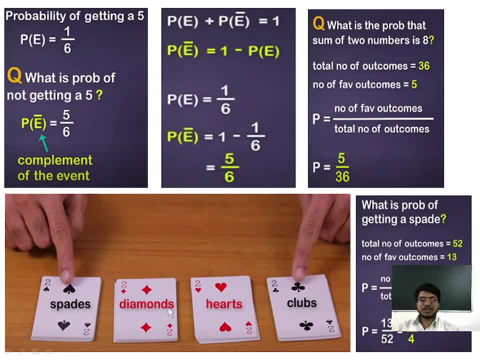 Now about deck cards. How many cards are there? 52 cards. are there Spades, diamond, heart club? What is the probability of getting a spade? Total number of outcomes is 52. And total number of favorable outcomes is 13 for spade Right. 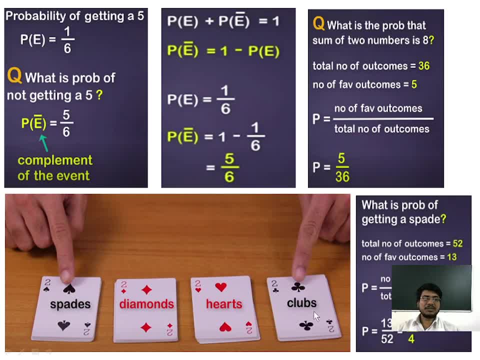 There are 13 spade cards, 13 diamond cards, 13 hearts and 13 clubs. So about spade, it is 13. And number of favorable outcomes are 13. Total number of outcomes are 52. So that is n a upon n again And you will get 1 upon 4. That is 25%. 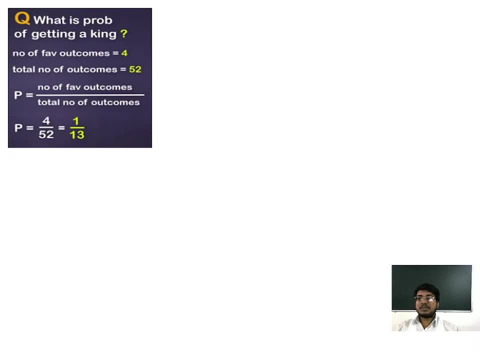 Now what is the probability of getting a king? Number of favorable outcome is 4.. About the king: Because 4 kings are in the 52 cards And possible outcomes are 52. So 4 upon 52, that is 1 upon 13.. 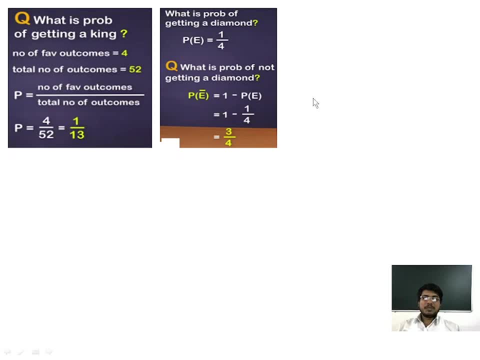 What is the probability of getting a diamond? So how many diamonds are there? That is nothing but 13 diamonds are there, as spade example. just we discussed. So you will get 25%. What is the probability? What is the probability of not getting a diamond? That is 1 minus this, 1 by 4.. That is 75%, 3 by 4.. 0.75. 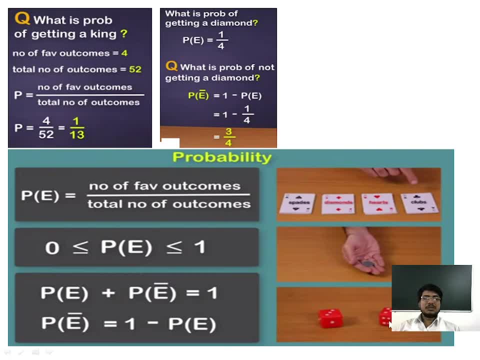 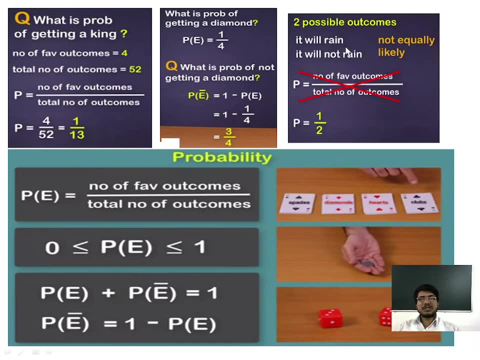 Now here we can summarize these examples we had just completed. Now, about the rain, There is uncertainty. We cannot say it will rain or it will not rain, So probability is not applicable in that case. When there is a uncertainty Not equally likely, When uncertainty is like what? Not equally likely, So we cannot apply probability there. in this regard, 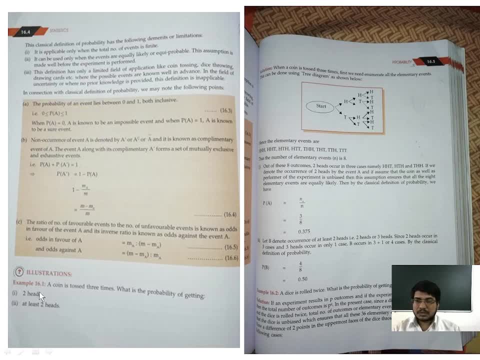 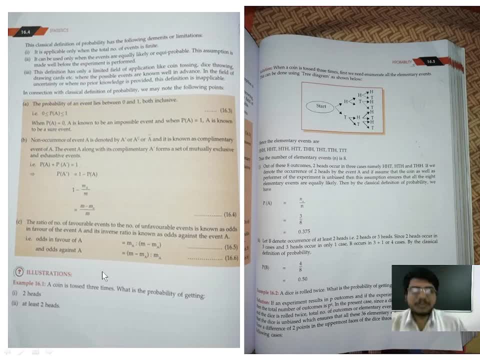 In last discussion I already given the explanation about how many times the coin is tossed. That is, you will take as a power to that 2 possibilities for a coin, 2 possible outcomes for a coin. So 2 raise to 3.. For a coin there are 2 possibilities, So that is 2.. And you will toss it is for 3 times. So it is 2 raise to 3.. So your sample space will come what 8.. 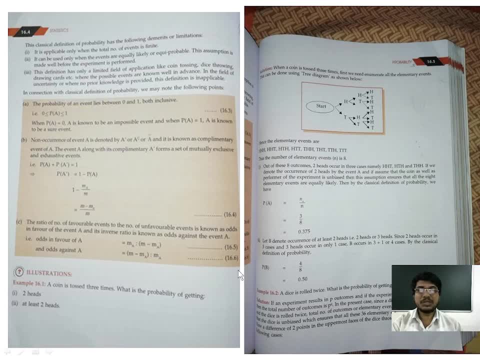 So your sample space will come what 8.. So your sample space will come what 8.. Please listen this carefully: 2 raise to 3 is nothing but what 8.. And that is nothing but sample space. That is n. 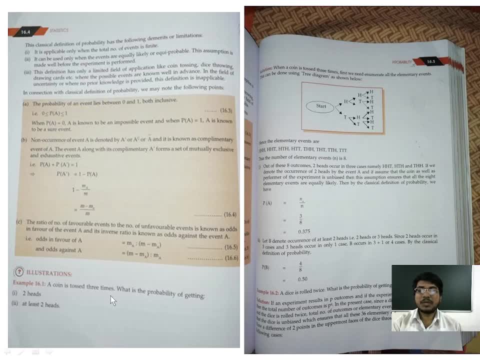 And they are asking 2 heads. So what is the favorable outcomes for 2 heads? So you will make the set here and you will find it is 3.. At a time you will get 2 heads are there and that are 3.. 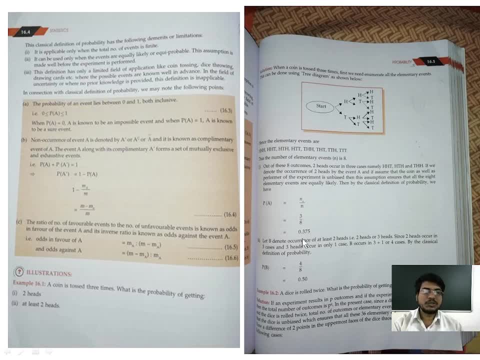 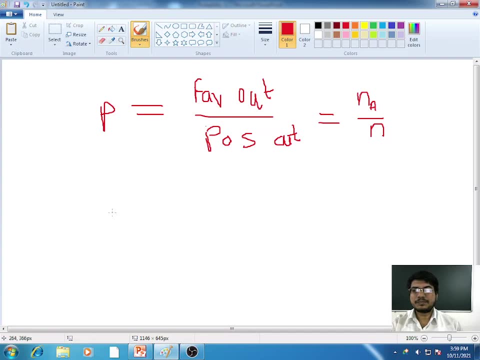 Okay, So your probability is 3 upon 8.. That is 0.375.. You can got it in this example. likewise, You can prepare this n a likewise. Or you can write this e. So for 3 times you are doing the experiment. So head, head, head will come. 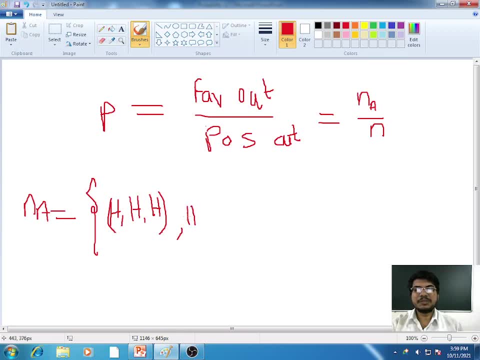 Right. So in this regard, you will prepare this: Head, tail, head, Then head, tail, tail. Okay, Then a tail, head, head. So likewise, you will going to prepare it and you will get answer 3.. 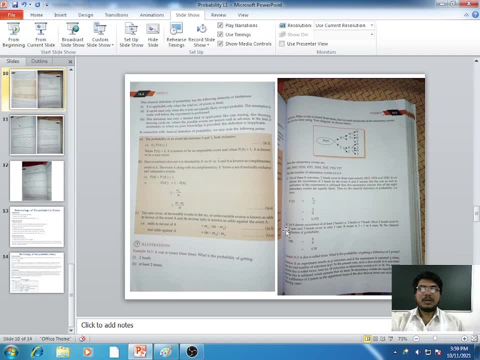 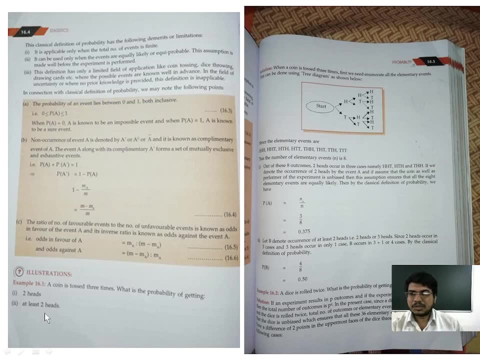 In our last discussion. just we completed that one, So I think you not find it is difficult. 3 will come there For 2 heads. Now next condition is asked for at least 2 heads. At least means what More than 2 heads are allowed. 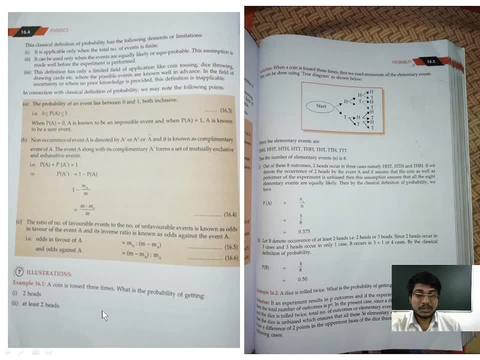 But 2 should be there. 2 should be there. In this regard, you will go through this chart. just, we had chart means this one or the set made by you, So that will come 4.. At least 2 heads, So that will come 4.. 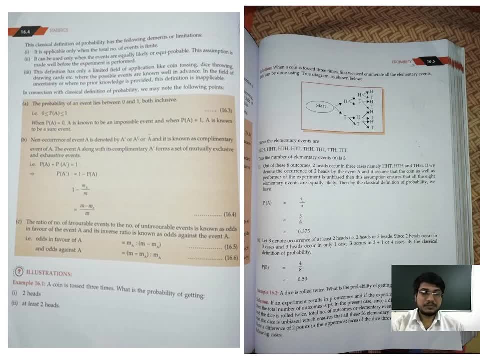 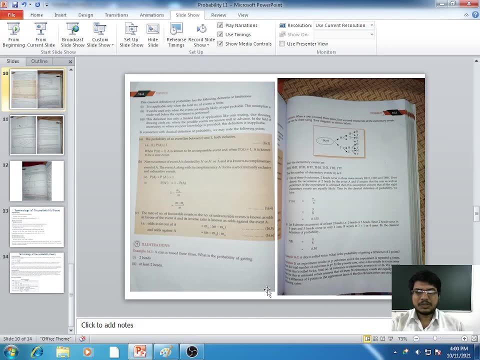 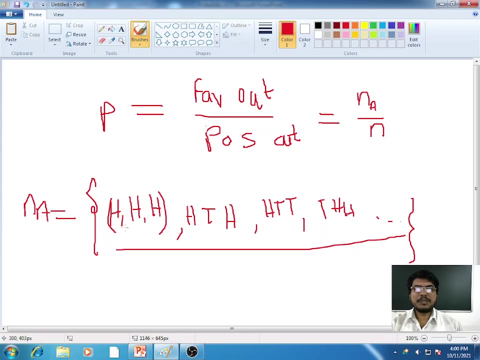 The probability of that event is nothing but 50 percent. Okay, So it is just challenging. you will try to. we can say, make the set about the condition given to you And then it is possible to you. Okay, this one. If it is capable to you how to write, then definitely you will write the number of favorable outcomes, number of favorable outcomes and possible outcomes. Okay, 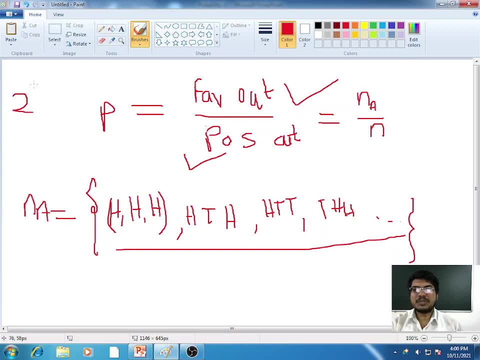 As 1 coin is there, we were getting two possible outcomes. One is available, The other is normal or the other is not. We have to write for, is there? so two possible outcomes and it is tossed three times. so it is 2 raise to 3 and 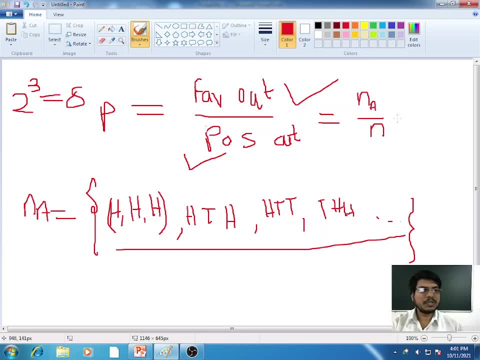 the possible outcomes are 8.. See, here will be what 8 and for first two heads are there. so once you will count that you definitely get three heads in that condition. So first answer is 3 by 8. but in the second condition they are asking at least two heads should. 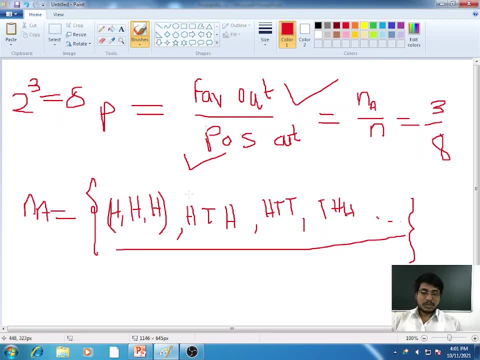 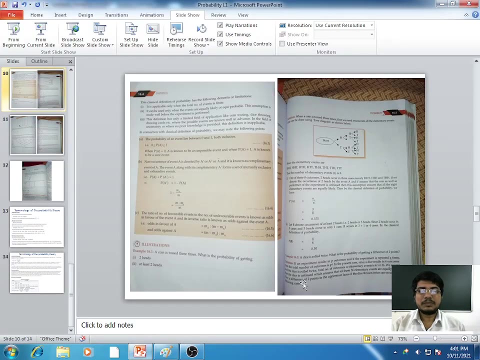 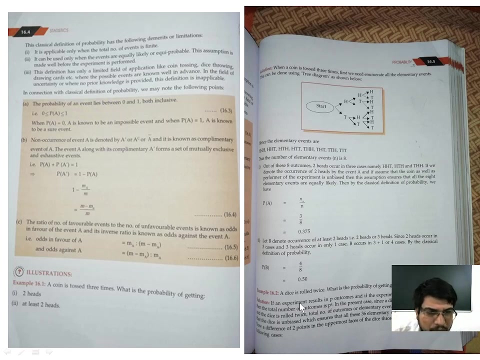 be there means more than two heads are also allowed. three heads are also allowed. So it will become what 4. it will become what 4, so 4 by 8.. Now see the next example. a dice is rolled twice. what is the probability of getting a difference of two point? 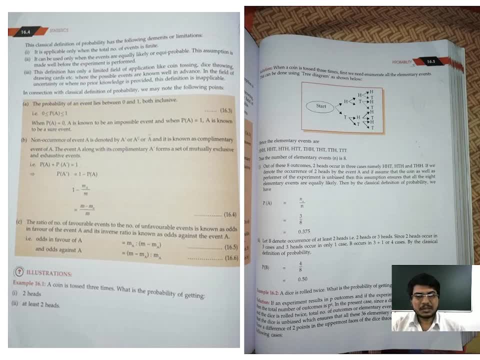 The example again is very simple. they are asking: a dice is rolled twice, a dice having six possible outcome. so 6 raise to 2, that will become 6, 6 or 36. so 36 is nothing but sample space, means small n. 36 is nothing but sample space. in our previous example we had 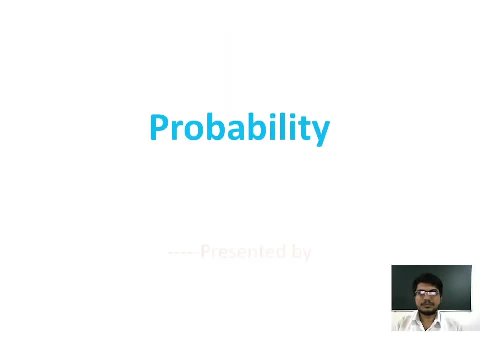 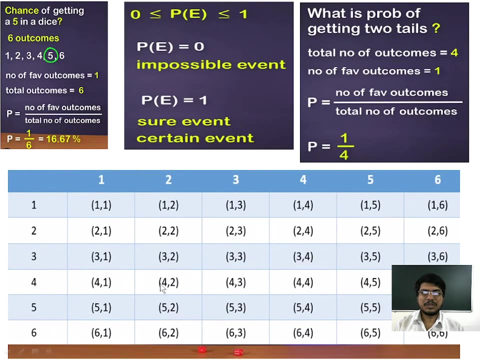 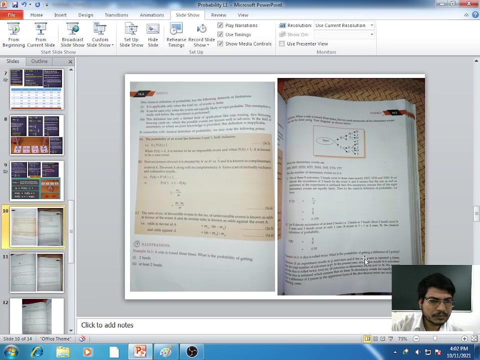 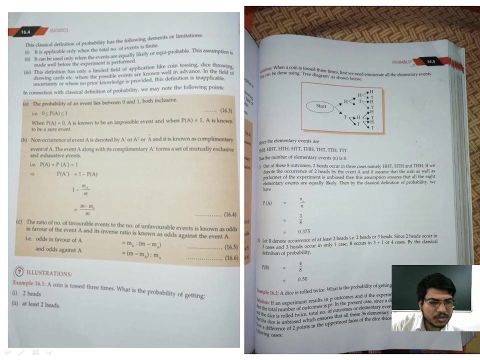 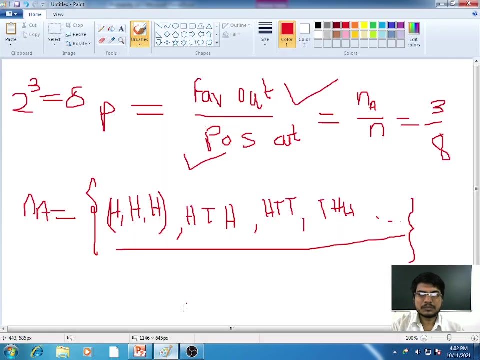 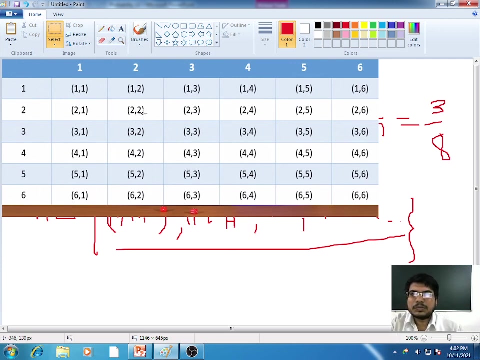 already. given that, Here it is, and they are asking difference of two points, getting a difference of two points in between them. so we will try, for the difference of two points will. So it is what? 4 minus 2.. It is there. Okay, This is one possible outcome. then, Again, you will try for another one. 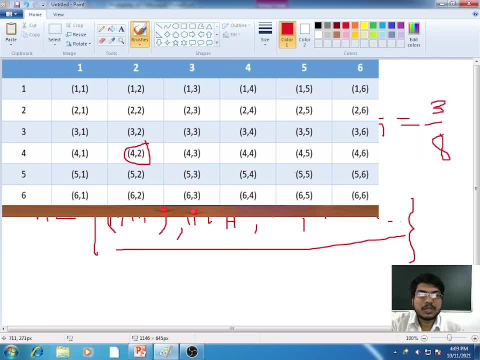 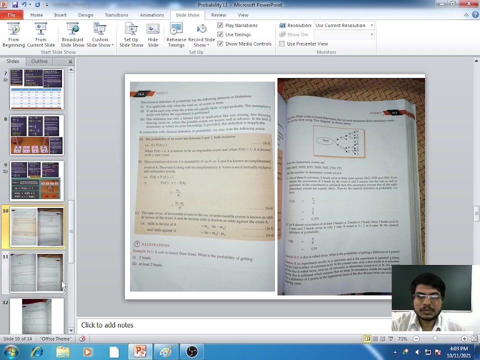 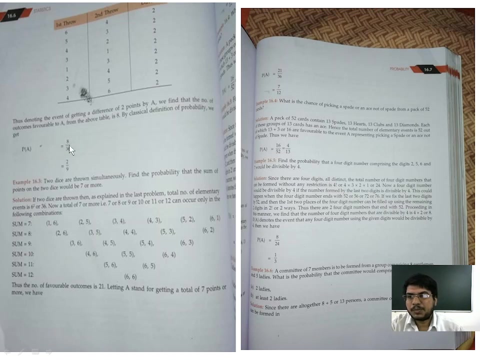 Now 5 minus 3,, 6 minus 4,, 3 minus 1.. So here you will get difference of 2.. Okay, There are another, maybe examples. Okay, So it is 8.. Number of favorable outcomes are 8.. Where the difference you are getting 2.. Again, we will check it. 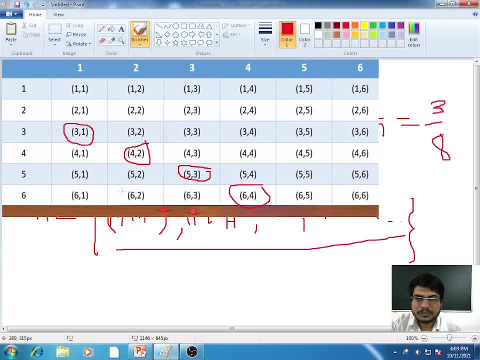 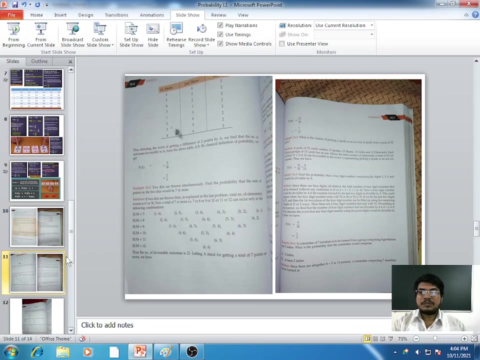 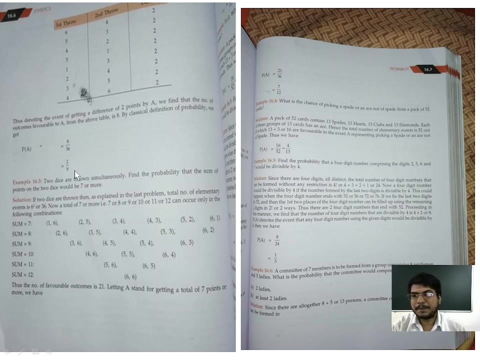 4 minus 2.. Then 1 minus 3.. 3 minus 5 and 4 minus 6.. Yes, So these are nothing but 8 possible outcomes. Others are not coming in this condition. So 8 favorable outcomes will come. So it is your answer: 8 upon 36.. So it is 2 upon 9.. 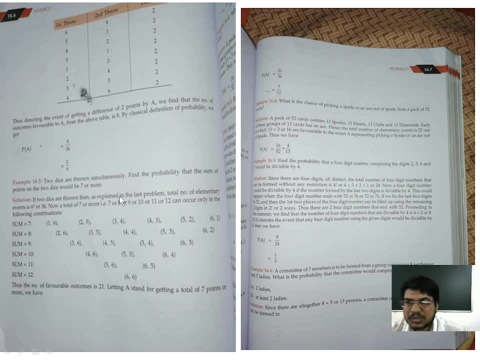 See the another example: 2 dice are thrown simultaneously. Find the probability that the sum of points on the 2 dice would be 7 or more? They are asking in the same way, But the condition is just changed. That sum of the points on the 2 dice would be 7 or more. We will try it. 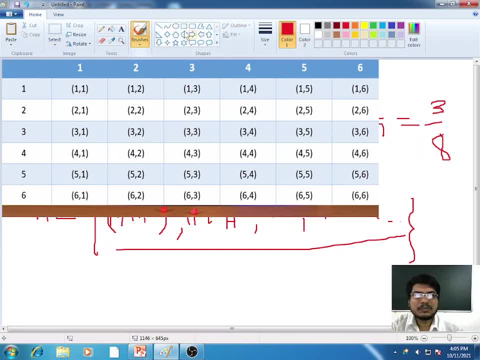 So 7 or more. the condition is there: 6 plus 1.. 7 is allowed, So it is all will come. Ok. So these all 6 will come, Then 5 upon 2 and this 5 plus 3, this will also come, Then 4 plus 3.. This will again come. This will again come. Yes. 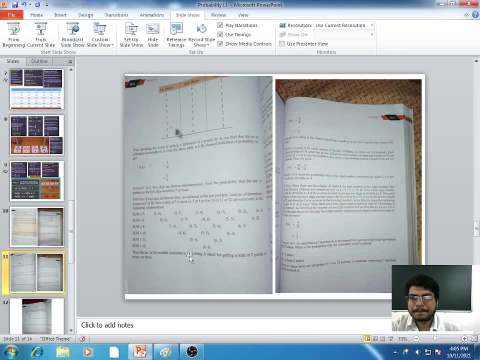 Again. we will come to the example. 2 dice are thrown simultaneously. Find the probability that the sum of points on the 2 dice would be 7 or more. They are asking in the same way: 2 dice are thrown simultaneously. Find the probability that the sum of points on the 2 dice would be 7 or more. We will try it. 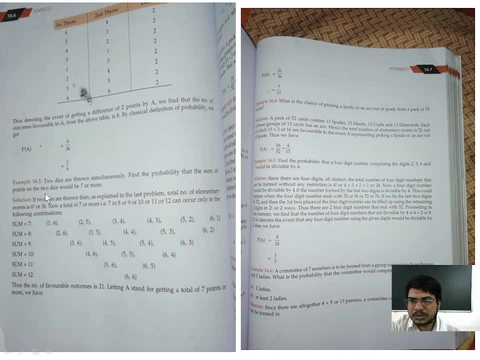 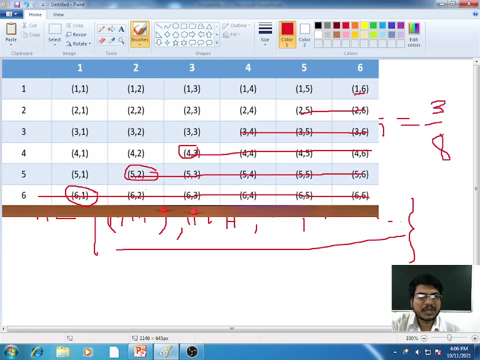 simultaneously find the probability that the sum of points on the two dice would be seven or more. okay, so in that regard, how many count will become just? you have to check it for favorable outcomes. 1, 2, 3, 4, 5, 6, 7, 8, 9, 10, 11, 12, 13, 14, 15, 16, 17, 18, 19, 20, 21. so there are 21 favorable outcomes, are there? 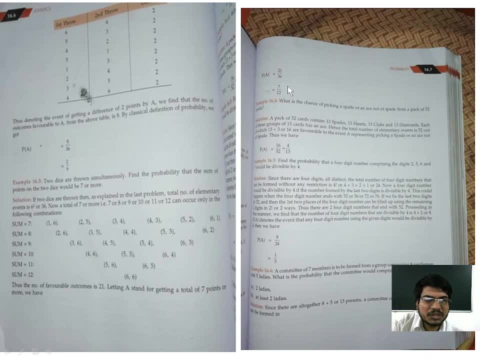 21 upon 36, so it is nothing but 7 upon 12 once simplified. so we can solve this example in this regard, just using the formula of probability and you will get the answers. thanks for patience listening. 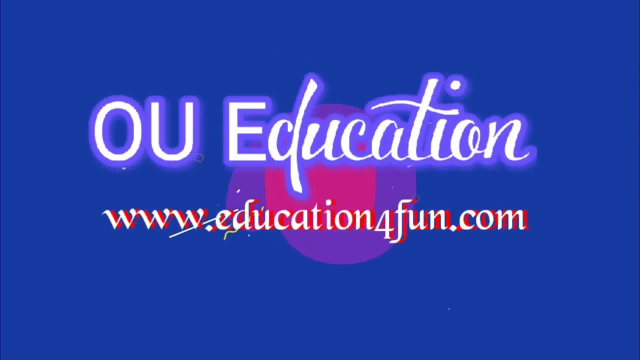 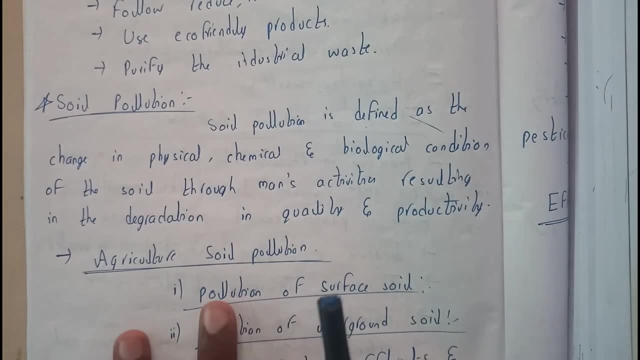 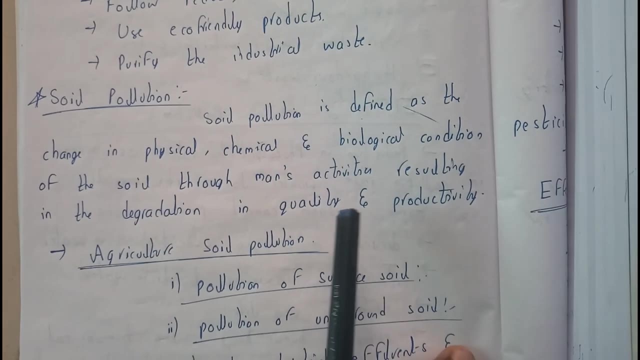 So, guys, we are back with our next tutorial. In this tutorial, let's see all about soil pollution. In the previous tutorials, we have learnt all about marine water and air, So in this tutorial, let's see what is soil pollution. 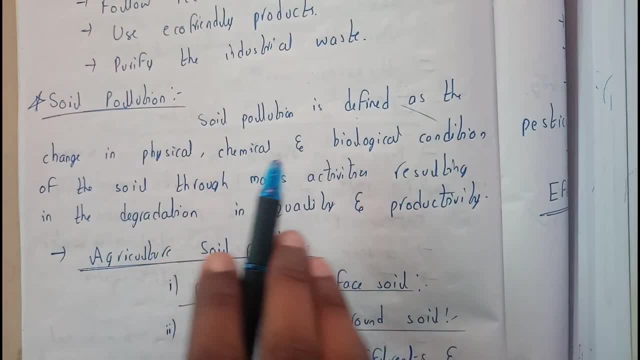 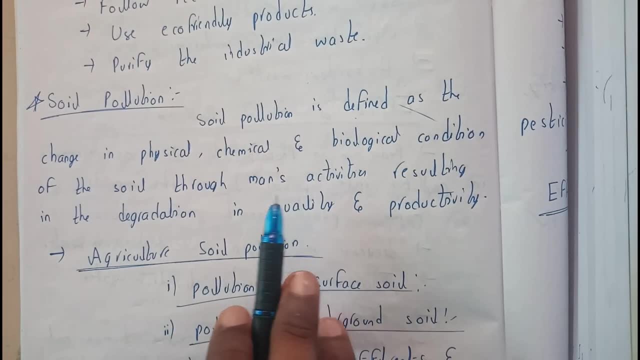 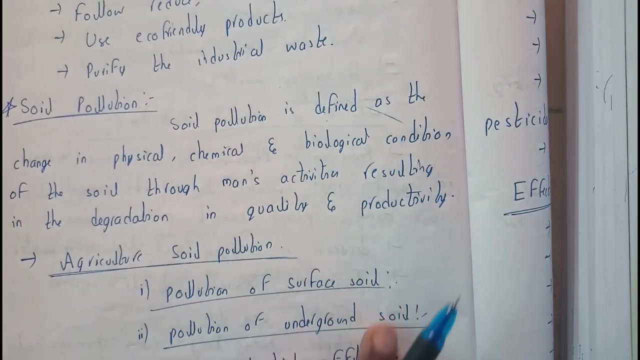 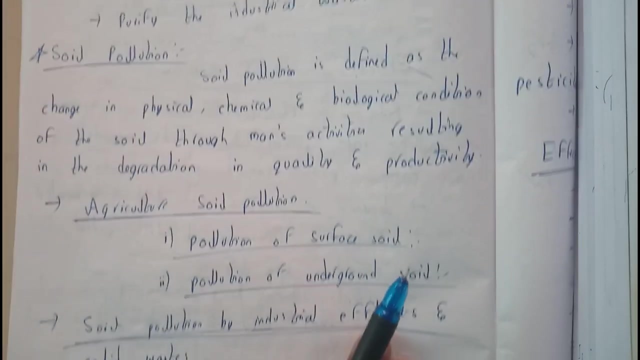 Soil pollution is defined as the change in physical, chemical and biological conditions of soil through man activities resulting in degradation of quantity, quality and productivity of soil. Basically, soil pollution is caused by many factors, guys. There is not one or two. Even there are many causes. Let's check out types of soil pollution. 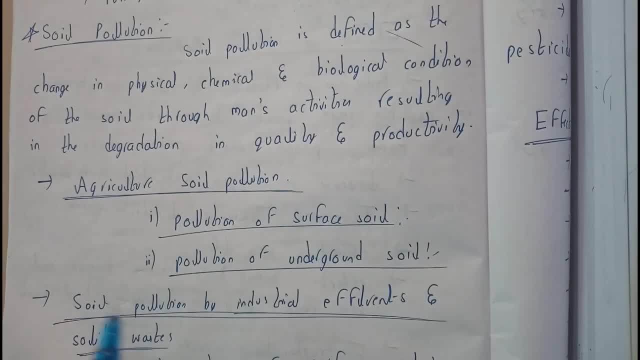 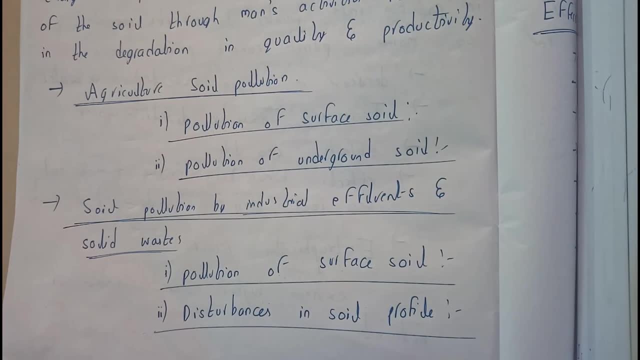 It is basically divided into two types, mainly Agricultural soil pollution and soil pollution due to effective wastes or something like that. Basically, I didn't write any examples here, So let's try to write some examples on them. Okay, let's go through them. 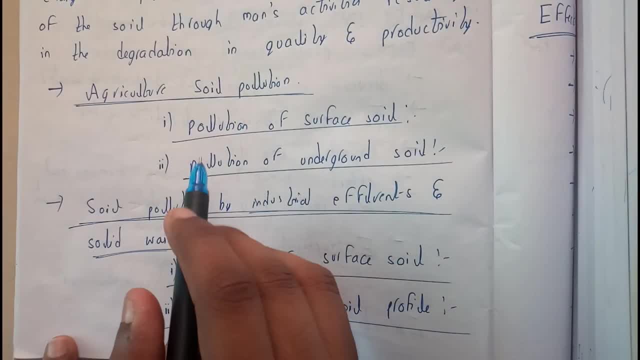 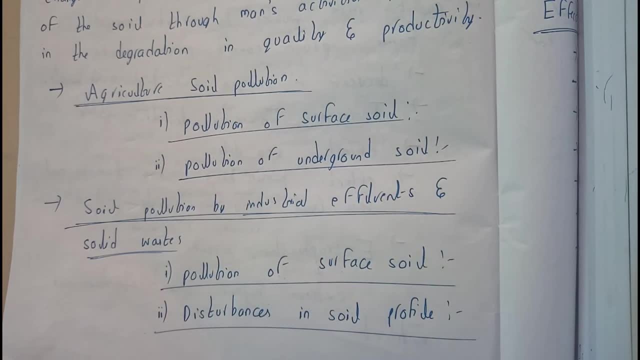 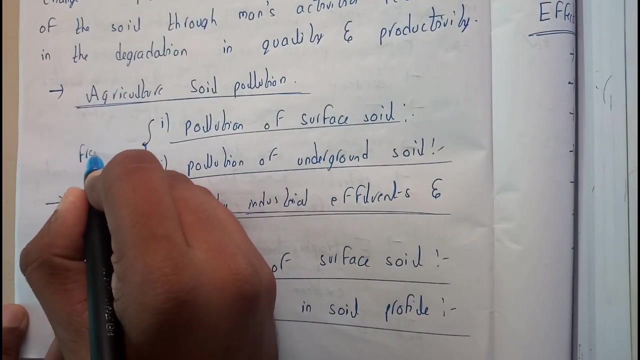 Basically, let's go through agricultural soil pollution. Agricultural soil pollution, Pollution of surface. Pollution of surface soil: Okay, surface soil can be polluted by these. both include usage of fertilizers and pesticides. guys, to be clear, Even it causes surface pollution and it causes 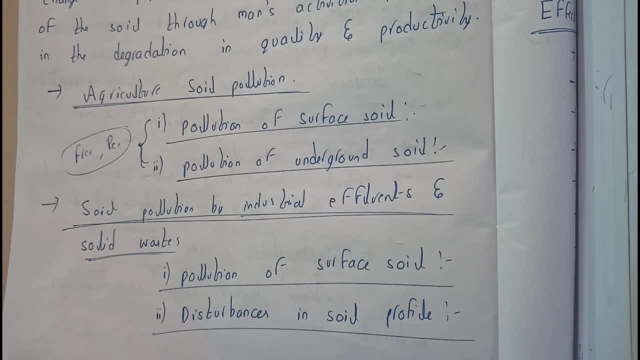 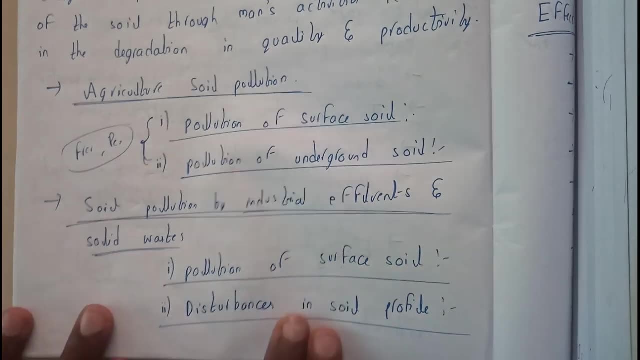 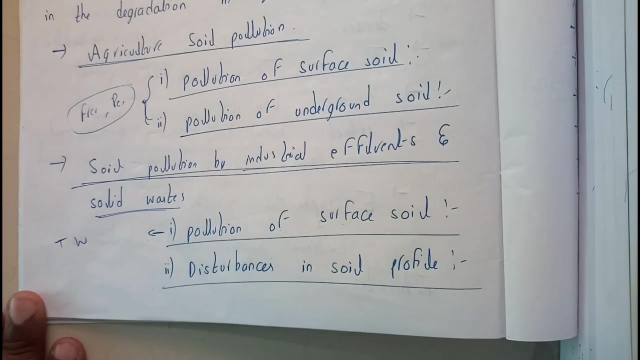 underground pollution, underground of underground, of soil. There are lots and lots of pollution guys. Whenever we go to industries, For industries, it is going to be for surface. It is just throwing off of waste materials, Waste materials which are unwanted waste materials. 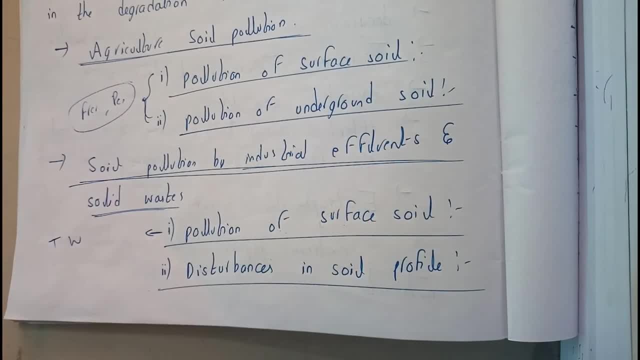 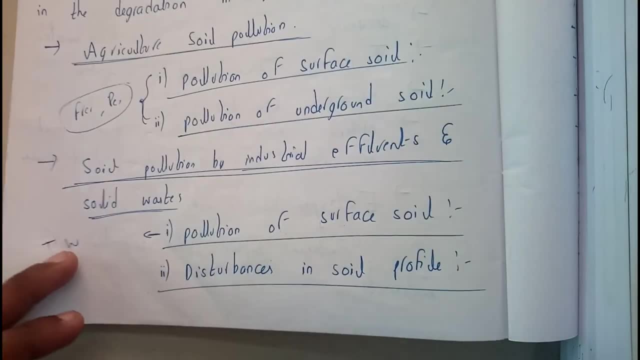 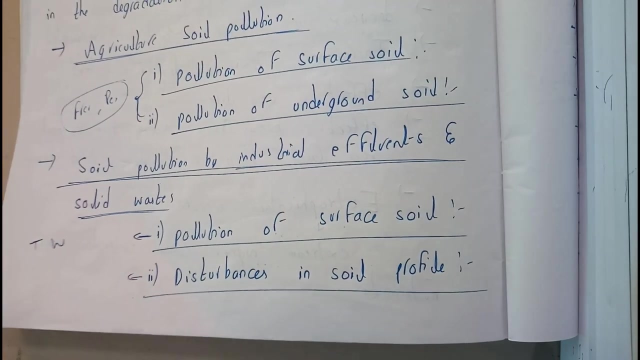 If we just throw them off on the surface of the soil, it causes pollution and internal pollution it includes. it may be due to the industrial wastes, like chemicals, which can easily damage the soil, and they can enter into the soil and damage a lot, even interior parts.